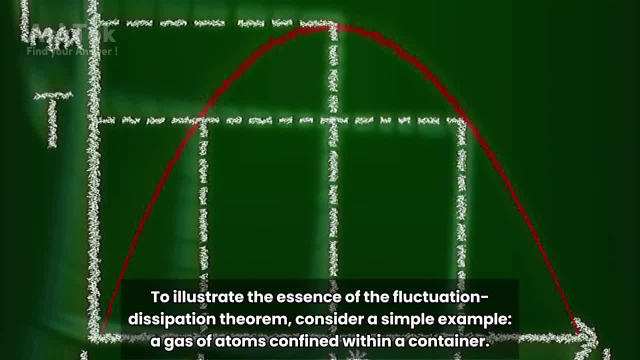 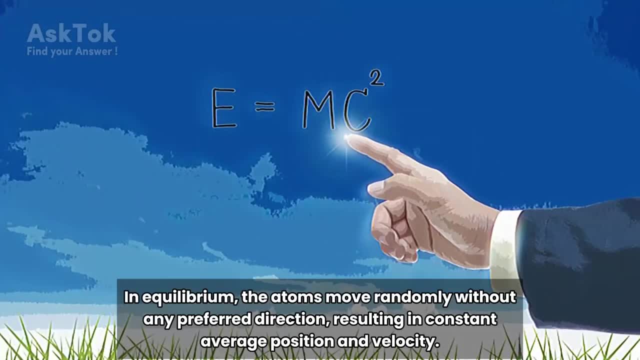 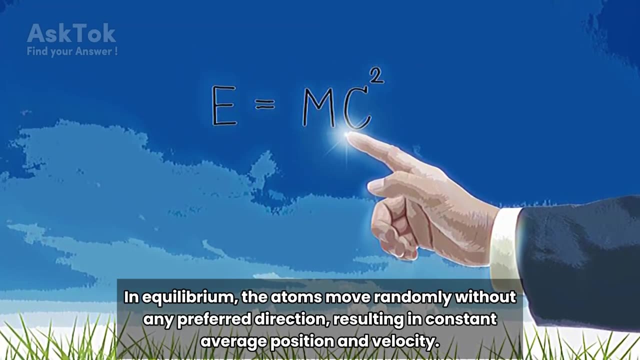 surroundings. To illustrate the essence of the fluctuation-dissipation theorem, consider a simple example: a gas of atoms confined within a container. In equilibrium, the atoms move randomly without any preferred direction, resulting in constant average position and velocity. However, 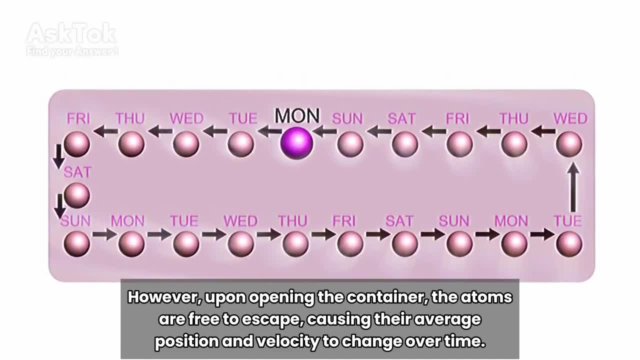 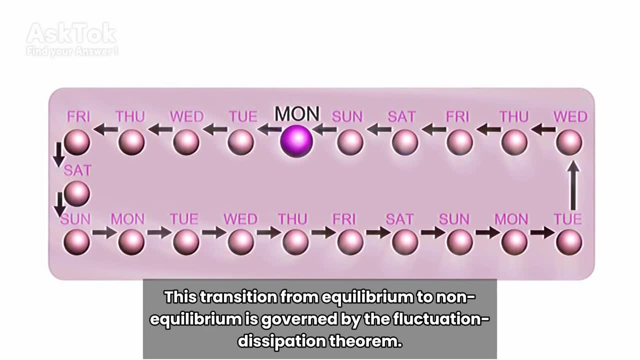 upon opening the container, the atoms are free to escape, causing their average balance to be less than or equal to the average balance of the atom. This is a very important example that illustrates the importance of the fluctuation-dissipation theorem. This transition from equilibrium to non-equilibrium is governed by the fluctuation-dissipation. 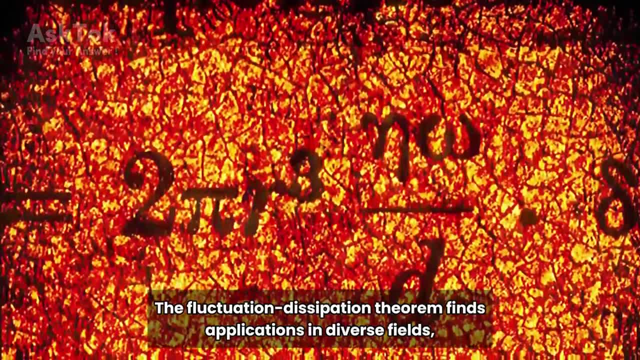 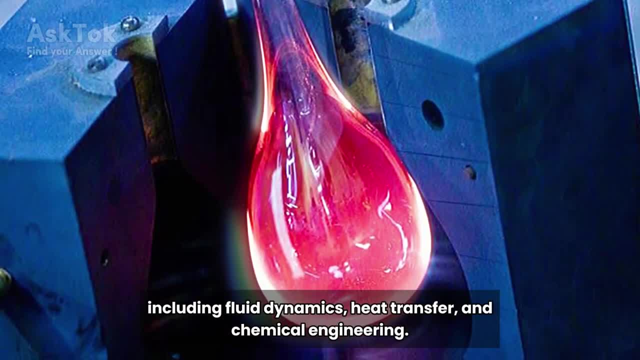 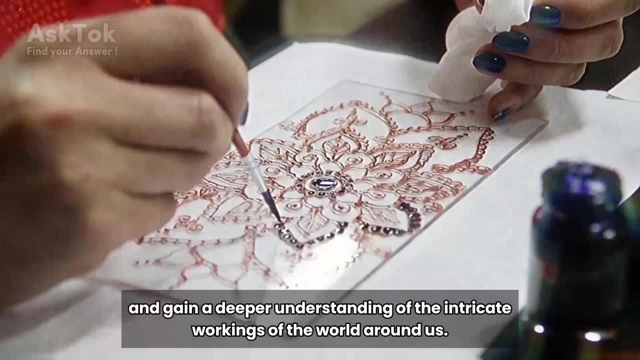 theorem. The fluctuation-dissipation theorem finds applications in diverse fields, including fluid dynamics, heat transfer and chemical engineering. By harnessing this theorem, we can design materials and devices with enhanced performance and gain a deeper understanding of the intricate workings of the world. 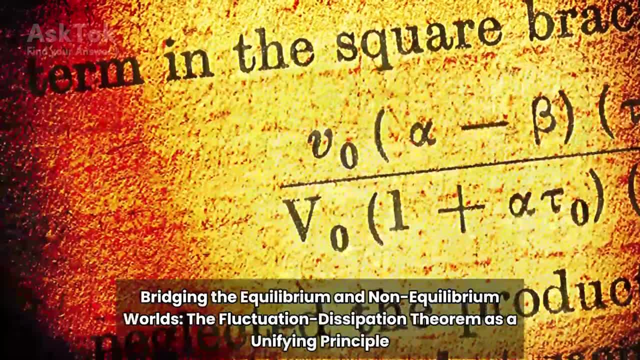 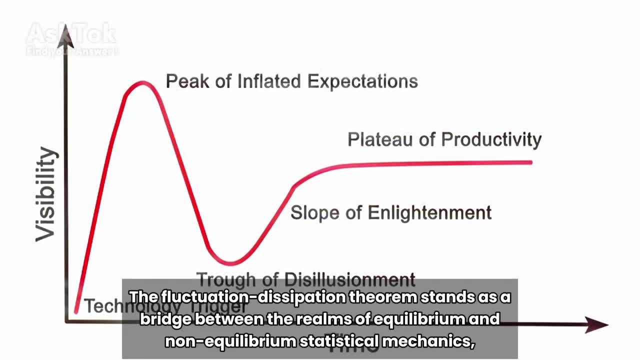 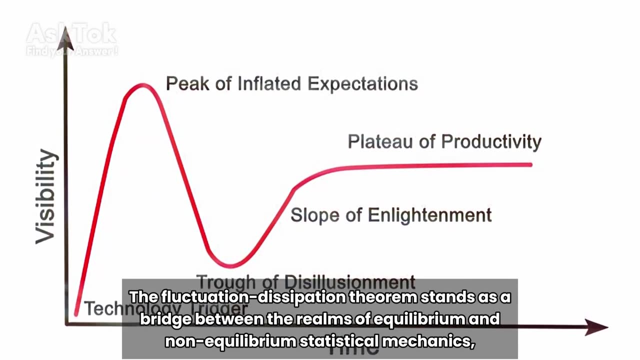 the world around us, Bridging the equilibrium and non-equilibrium worlds. the fluctuation dissipation theorem as a unifying principle. The fluctuation dissipation theorem stands as a bridge between the realms of equilibrium and non-equilibrium statistical mechanics, Revealing a fundamental 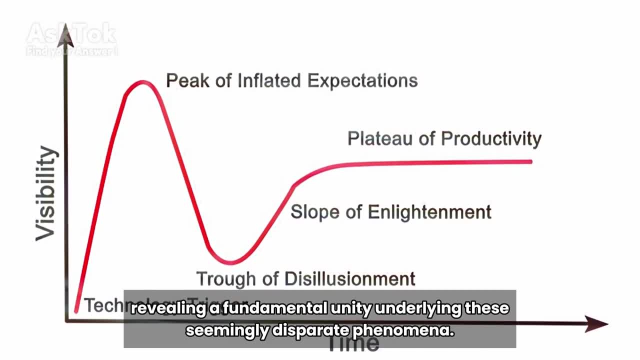 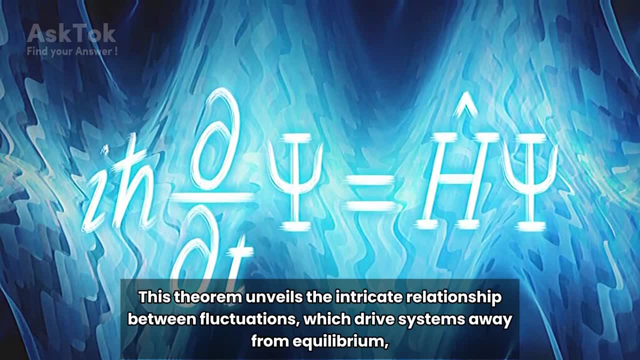 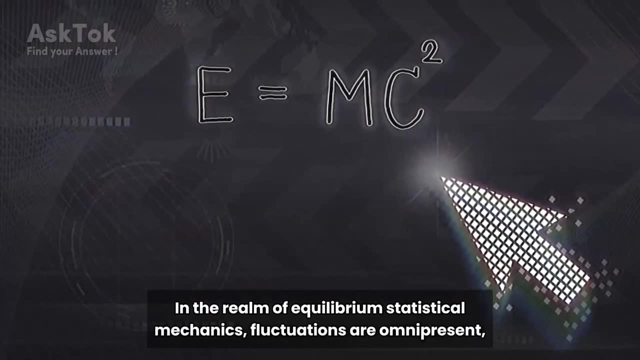 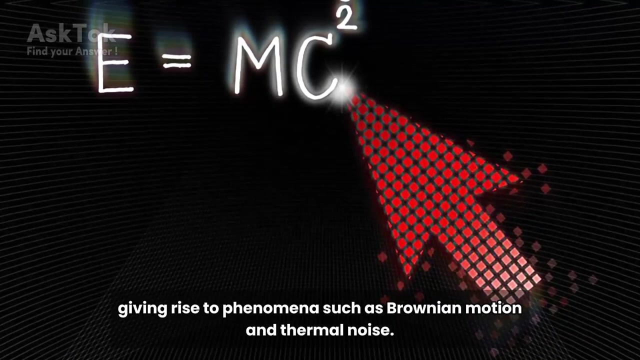 unity underlying these seemingly disparate phenomena. This theorem unveils the intricate relationship between fluctuations, which drive systems away from equilibrium, And dissipation, which counteracts these fluctuations and restores equilibrium. In the realm of equilibrium, statistical mechanics, fluctuations are omnipresent, Giving rise to phenomena such as Brownian motion. 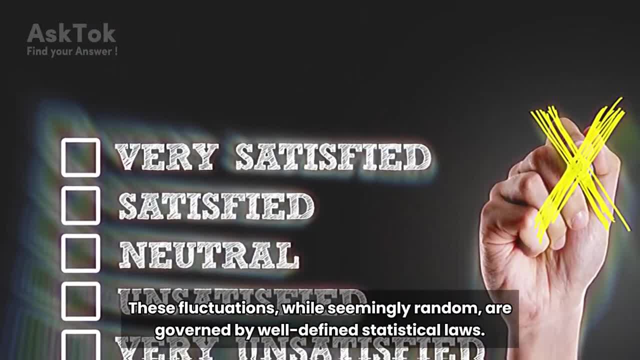 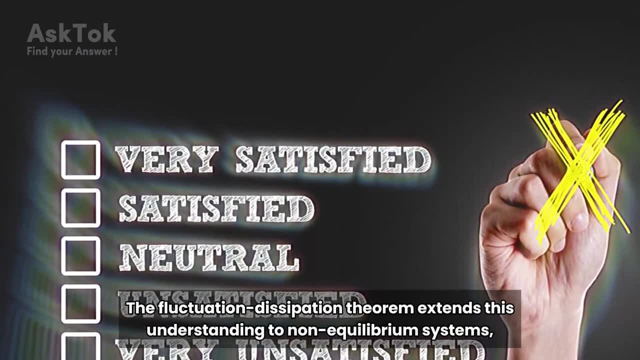 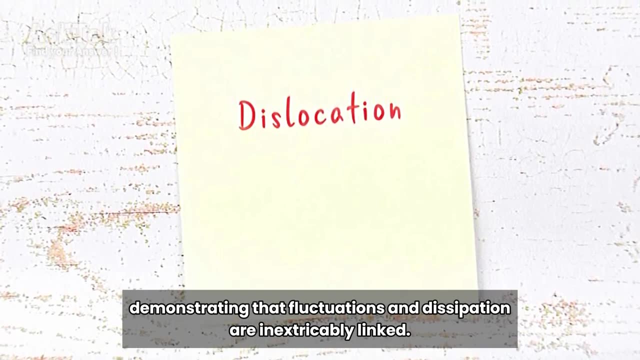 and thermal noise. These fluctuations, while seemingly random, are governed by well-defined statistical laws. The fluctuation dissipation theorem extends this understanding Understanding to non-equilibrium systems, Demonstrating that fluctuations and dissipation are inextricably linked. The fluctuation dissipation theorem has far-reaching implications. 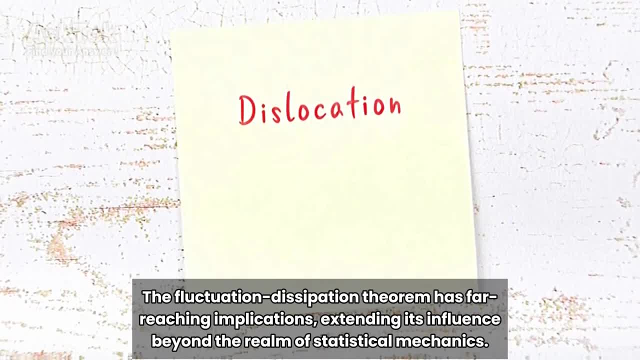 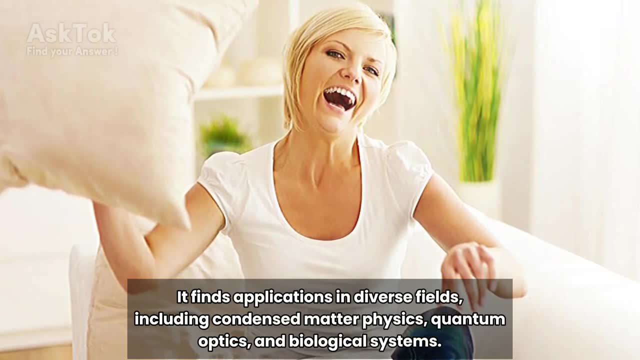 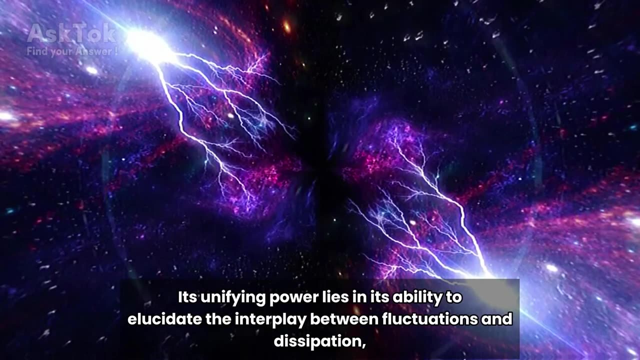 extending its influence beyond the realm of statistical mechanics. It finds applications in diverse fields, including condensed matter physics, quantum optics and biological systems. Its unifying power lies in its ability to elucidate the interplay between fluctuation and dissipation, Providing a deeper understanding of complex phenomena across a wide range of